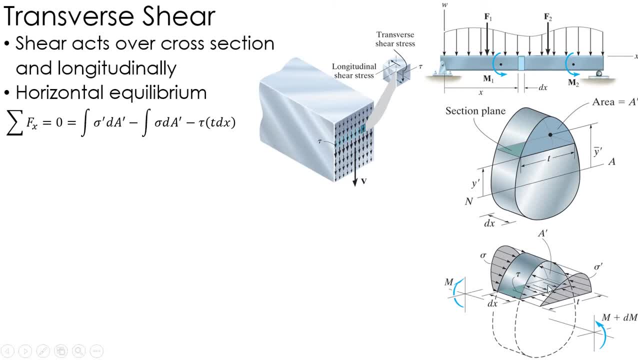 eat. No, I'm sorry. the stress on both sides plus the shear stress on that cut surface have to equal zero, and that's essentially what I have here. Okay, where I have sigma prime, dA prime, sigma dA prime, where A prime is the area above where I'm. 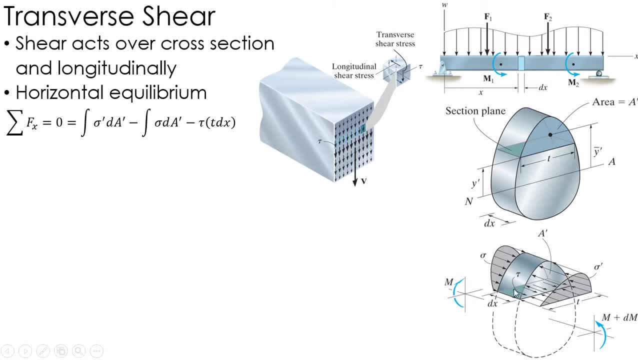 considered looking at the system, And then that's got to equal tau times the area down here which is Tx times, basically the width across where I cut it at T. So I'm manipulating this a little bit. okay, And using our flexure formula we used previously, I can find those normal stresses relative to the 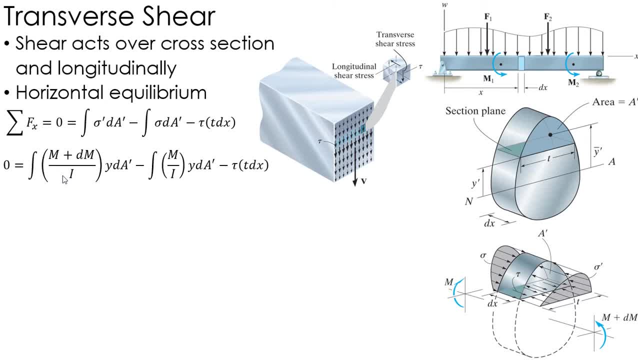 moment stress by essentially My over I and that's what I have here. So I have d plus dm on this side and just m on this side. so that's what I have here And again, that's My over I. okay, and that's what. sigma equals times each of the dA's- okay. 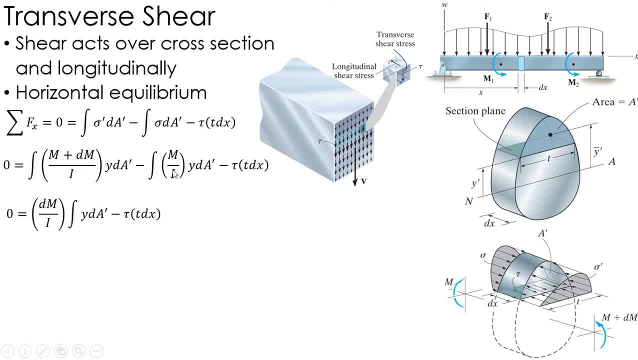 Well, what happens here is the m over I's cancel. I'm just left with dm over I. okay, Which is going to be constant relative to my area. here It is not constant relative to the x-axis, but relative to the area over which I'm integrating. right. 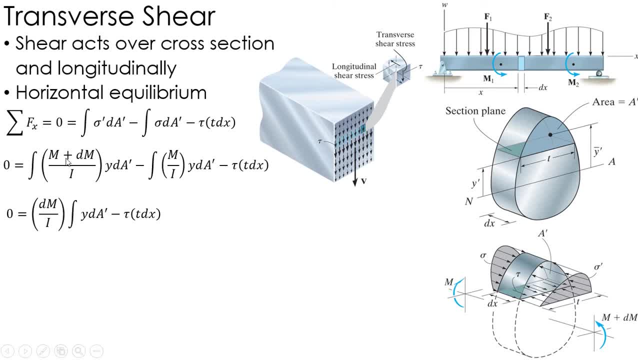 I'm integrating over this area. okay, That moment is constant, so I bring that outside as so. Now, solving this for my shear force or shear stress, which again is on this flat surface that I've cut. okay, I get the following: 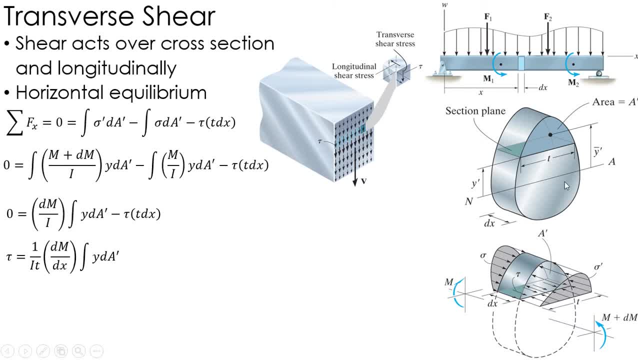 Pulling out everything that's constant, which include the moment of inertia of the entire cross-sectional area T, which is the width at the location that I'm looking at. okay, Then I have dm dx- okay, just with the dx over here and I'm just left with this. then integral of y dA prime: okay. 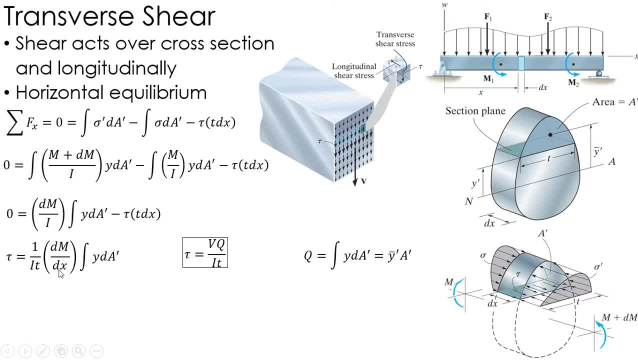 So here's what I've got: dm dx- you'll remember in our discussion- is actually V right, The derivative of the moment is my shear force, so I put that and then I lump all of this garbage here, this integral, and I call that the variable Q.